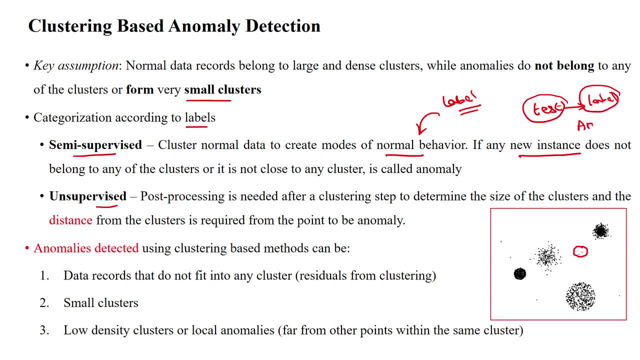 the label is not available, then that is called anomaly. if label is matching with the given data set labels, then that will be normal data point in unsupervised method. post processing is needed after your clustering step to determine the size of the clusters. here we will use the distance. 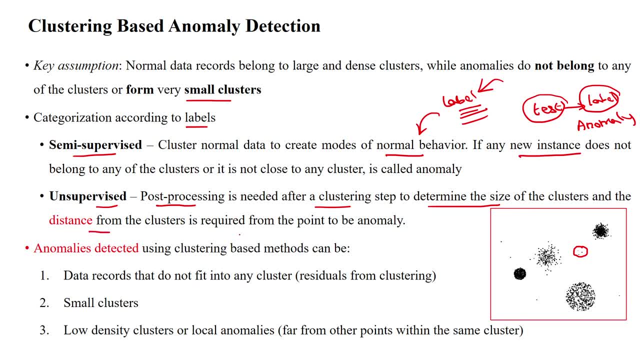 metric to measure the distance between two clusters. if any data point that is not available inside the Any aidade, adresina, piano, pesc, I mean the data point that is not available inside the any a did not other cluster, then that is called anomaly. data point anomalies can be detected by using various 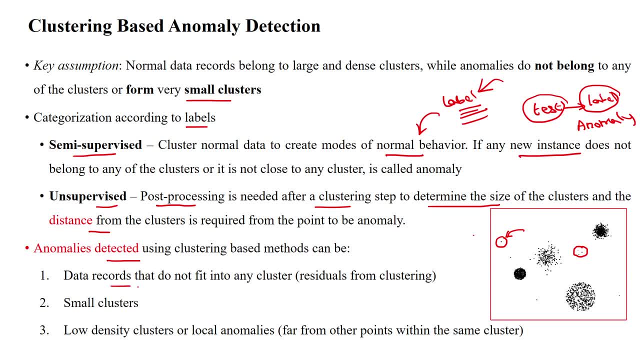 clustering methods. here the data points that do not fit into the any cluster is called residuals of cluster, so that will be called anomaly here. these data points are not belonging to any of the cluster, so these data points are called anomalies in the given data set and small clusters also considered as anomalies. for example, this is: this is having only three. 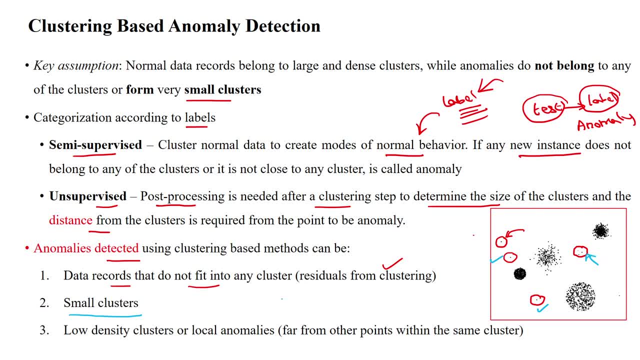 data points. this is very small cluster. that is also anomalies. and low density clusters are local anomalies. here the low density in the sense the data point with one or two or three. so these are all called low density data sets. that is also called anomalies in the given data set. so which? 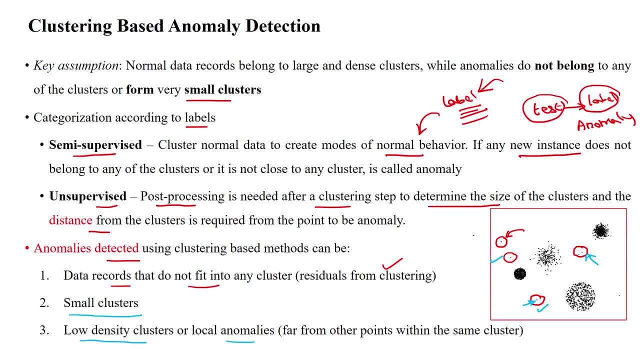 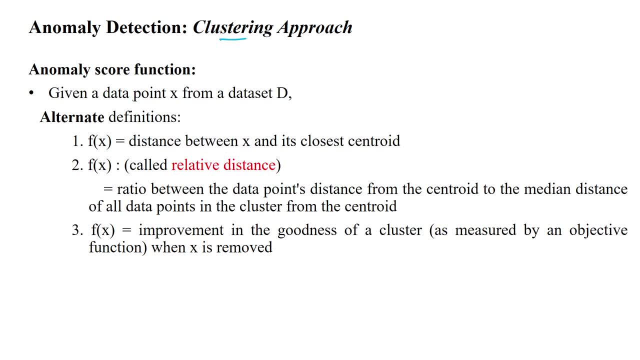 which pattern will be varying from the normal data points patterns. for detecting the anomalies from a given data set by using the clustering approach, we have to calculate the distance between the given new data point and its centroid. then if any data point is close to the centroid then that will be added. 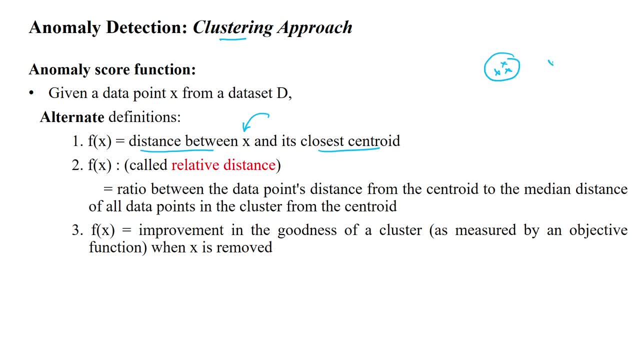 into that cluster. otherwise, if any data point which is far away from this centroid, if it is the centroid, if it is far away from the centroid, then that will be called an outlier or anomalies from the given data set. to improve the clustering size we have to use the distance metric for every iteration by calculating the new centroid. 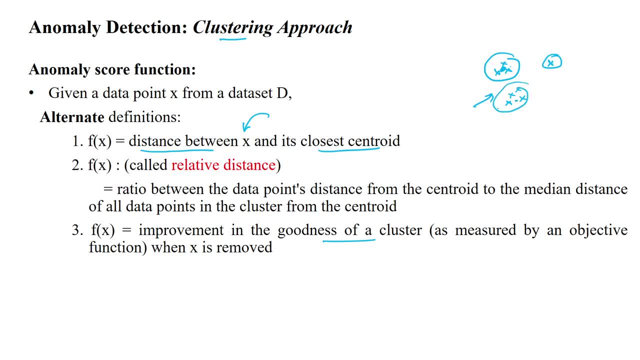 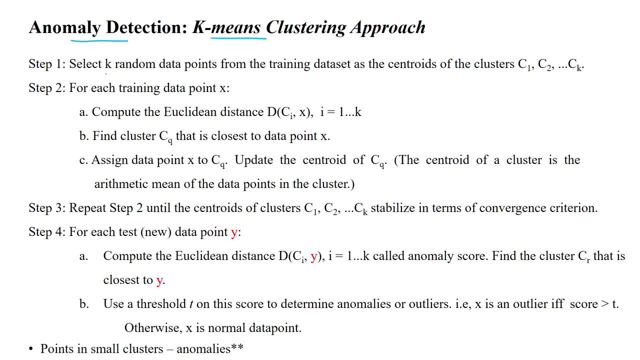 for each and every cluster that clusters given in the data set. here anomaly can be detected by using the k-means clustering approach. here initially we have to define the k number of groups or k number of clusters for defining the number of groups for given data set. so 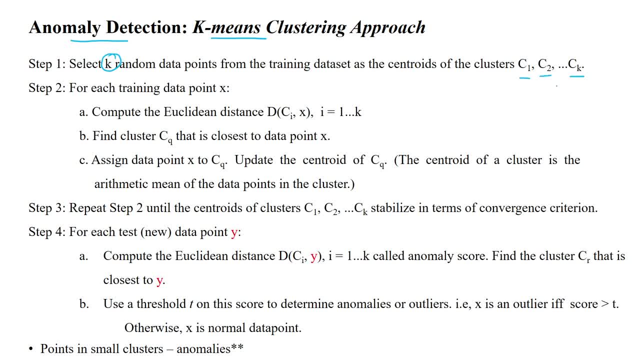 here k in the sense cluster, one cluster, two, k number of clusters. for each training data point x we have to compute the euclidean distance or the distance between the given data point to the centroid, then find the cluster centroid that is closest to the data point x. then if, 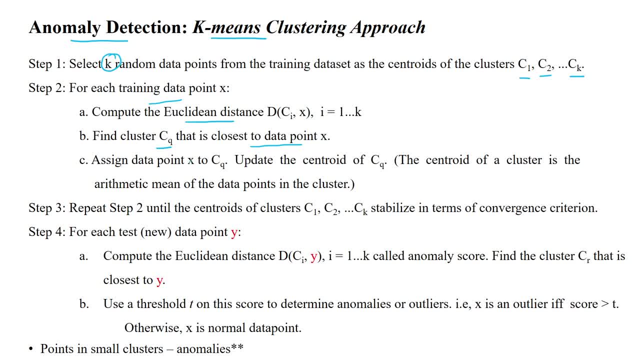 it is particular cluster, then we can assign that data point x into the closest centroid cq. then after performing that merging of new data points with the cluster, we have to update the centroid for this new clusters. so again we have to repeat the step 2 until centroids of the cluster are. 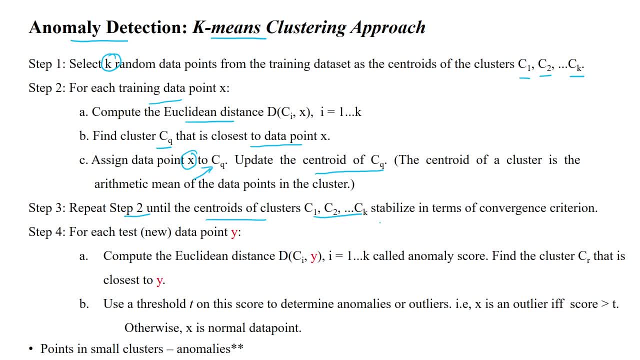 becoming stable. that means number of cluster centers should not be changed or number of data points should not be changed in the each and every clusters. that that criteria is called convergence, suppose. if i am having the number of data points here, so here centroid also should not be changed and a number of data points are available in the cluster also should not be. 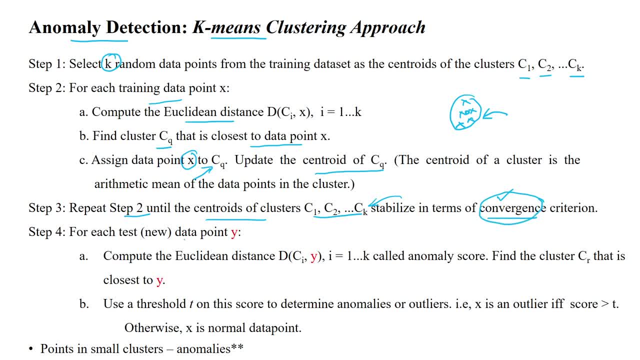 changed so that is called convergence criteria. for each test test, data point y, when it is coming into our model, we have to compute the Euclidean distance. suppose if I am having the three clusters here like this, then when I am getting the new data point y, so when it is coming to here here the cluster centers are there, so it will calculate. 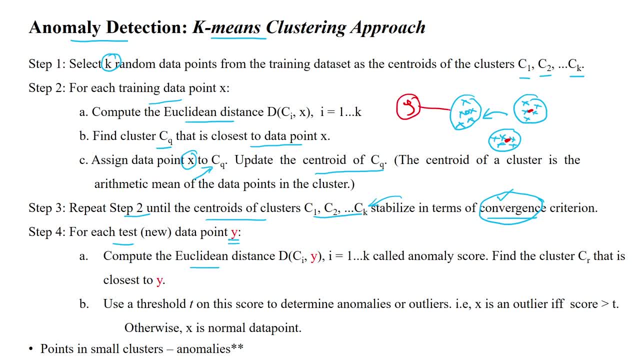 the y's data data points, distance from each and every cluster centroids, then whichever is close to this data point y, then that y will be added into that respective cluster. so here, if it is not belonging to any this pattern, any of this cluster pattern, then it will be called anomaly.